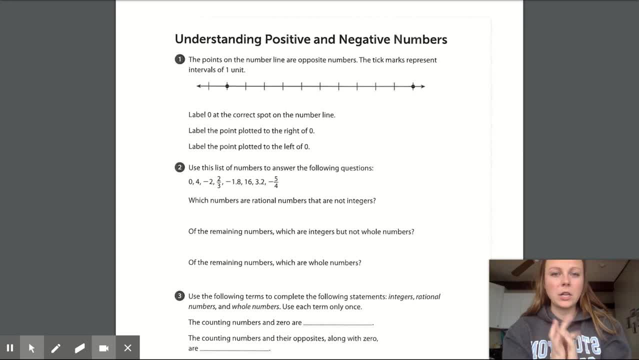 Opposite numbers are the same distance from zero, just on either side of zero. So knowing that these two dots are opposites, that's going to help us to figure out where zero belongs, because wherever I put zero, it should be the same distance between both points. 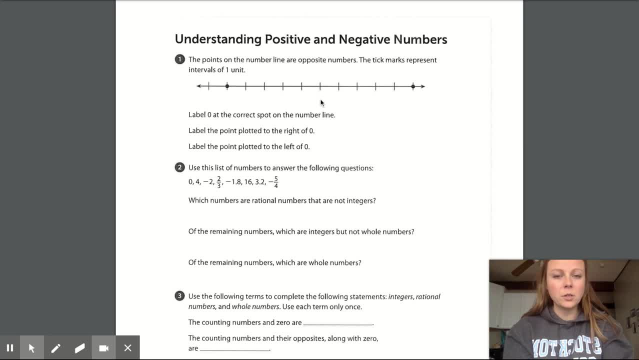 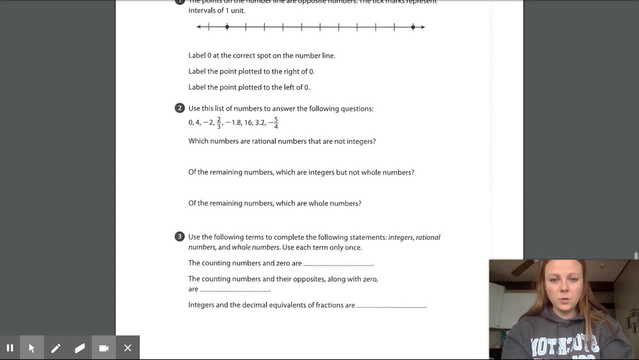 They also tell me that each mark is representing intervals of one. so once I find zero, I can label one to the right and negative one to the left. Number two: now they're going to go into what are rational numbers and what are integers. 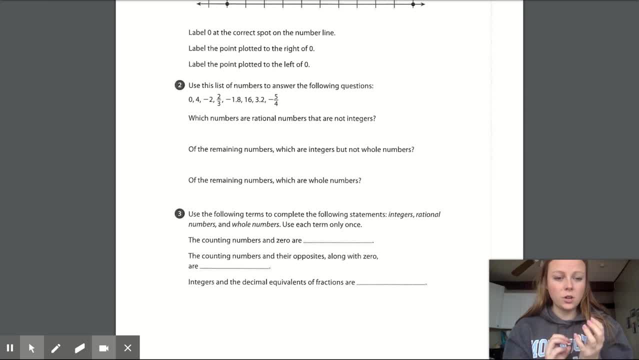 So two different categories of numbers. Integers are your whole numbers, so counting numbers one, two, three, four, five, The number zero, and all of those counting numbers opposite, so negative, one, negative, two, negative, three, negative, four. 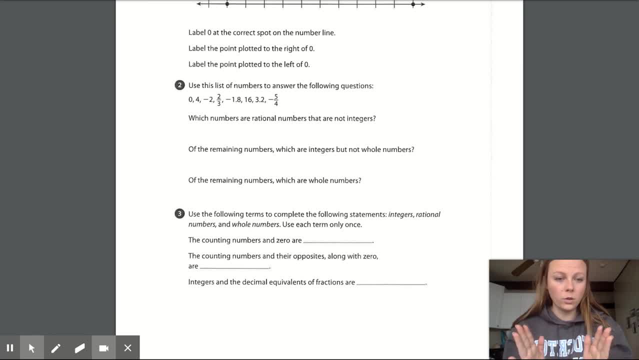 So no decimals, no fractions, all whole and counting numbers and zero Rational numbers are kind of all-inclusive: It's the fractions, the decimals, positive, negatives, So it's kind of like all the numbers we use. So integers are a little more exclusive. 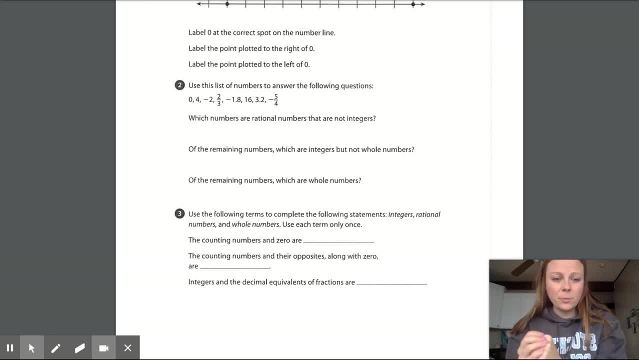 Rational numbers include a lot more. The only things that are not rational Rational numbers are irrational numbers, which we don't really use in sixth grade. It's things that are infinite, such as the number pi. It goes on forever and ever. 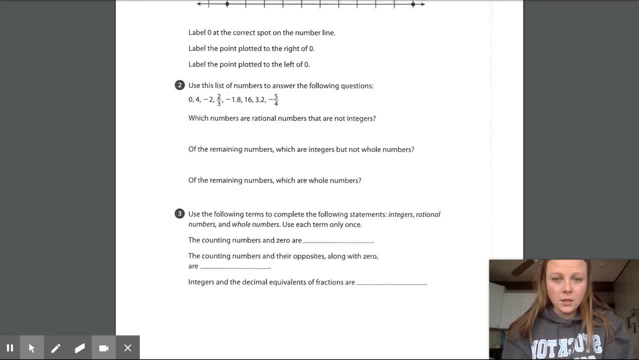 It doesn't have an end. So they're asking you to categorize the list of numbers: which ones are integers, which ones are not, which ones are whole numbers. So whole numbers, you know. no fractions, no decimals, All right. 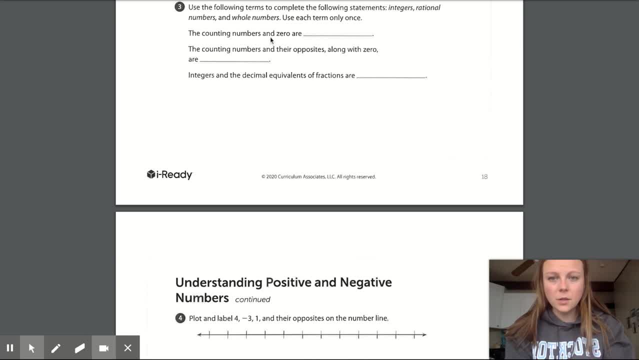 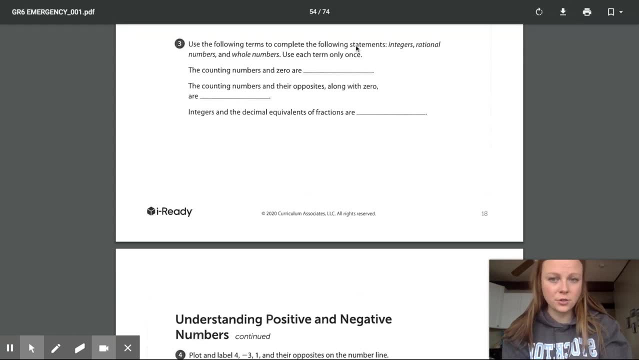 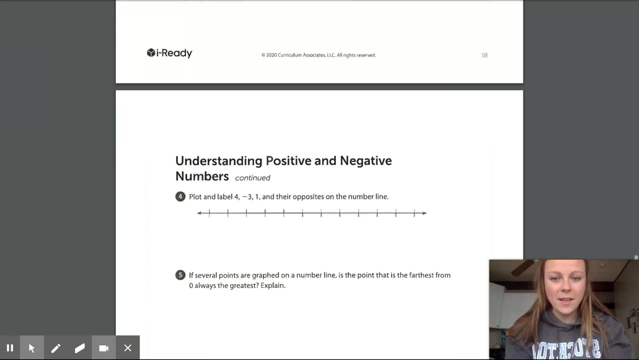 So again, just some more definitions, Counting numbers and zeros: is that an integer, rational number or whole number? If you get really stuck, you could Google the definitions of those and examples That'll help you. okay, Here you're plotting numbers on the number line. 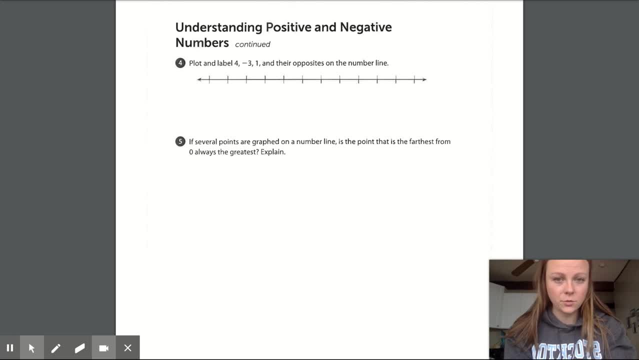 So you're going to plot the numbers and their opposites. So read that carefully. They're giving you tick marks. You're going to have to label it. I recommend putting zero pretty much in the middle, since we're dealing with both positive and negative.